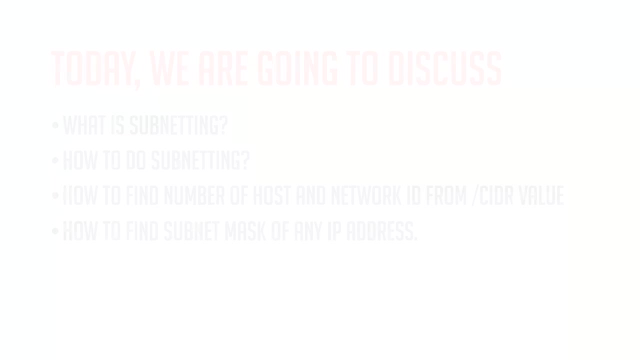 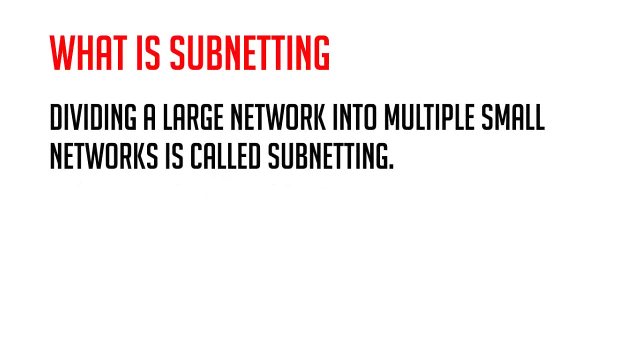 and welcome back to my channel, technical tech. Let's the tech begin. So, guys, what is subnetting? Dividing a large network into multiple small networks, we called it as subnetting. Before starting the concept subnetting, I would like to explain you about few basic things. 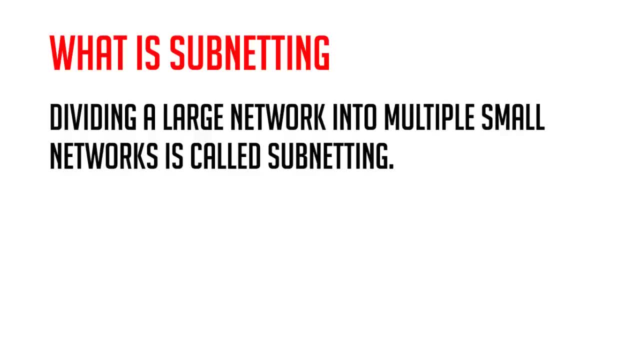 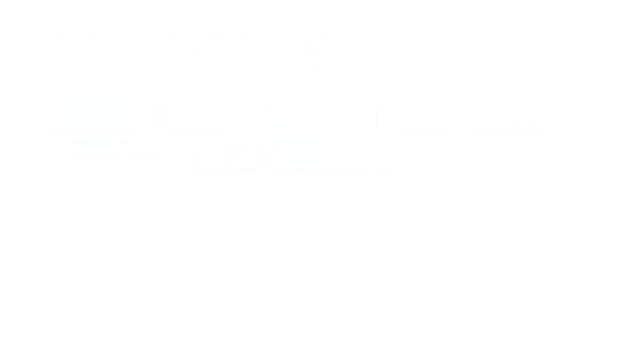 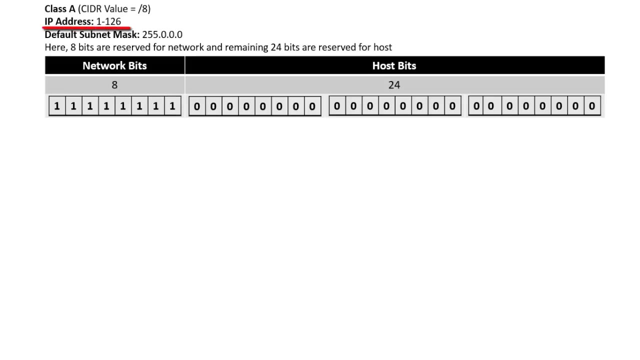 Because if you don't know the basic, it will be very difficult for you to understand the subnetting concept. So, guys, please follow the video, Watch this video till the end, then only your all the confusion and doubt will be clear. Let's start with the classes of IP address. As we know that class A IP address starts from 1 to 126.. 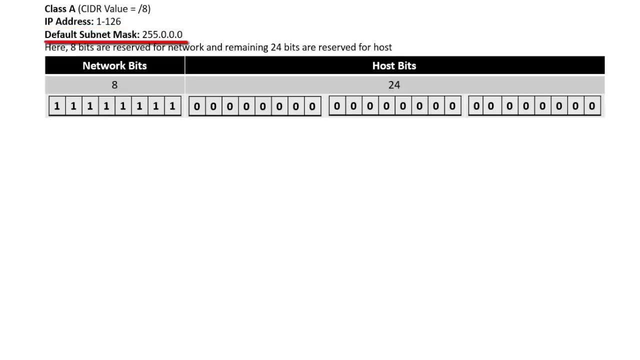 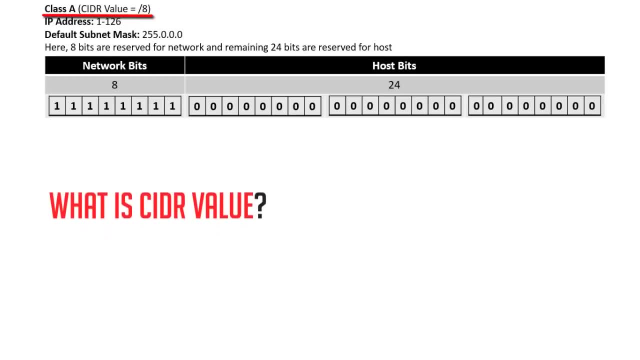 CIDR value means and why the default's CIDR value of class A IP address is 8.. CIDR stands for classless inter domain routing. It is the total number of network bits. As here you can see, in class A IP address there are 8 bits reserved for the network. 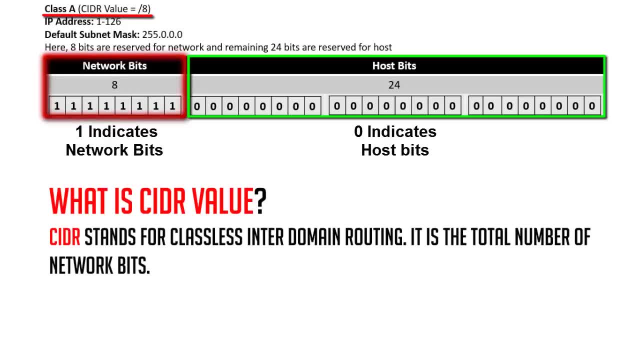 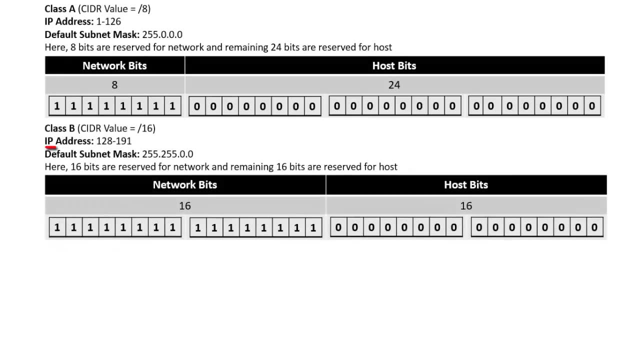 and the remaining bits are reserved for the host. So this 8 network bits is a CIDR value. That's why the default CIDR value of class A IP address is 8.. Now let's move on to class B. Class B IP address starts from 128 to 191. 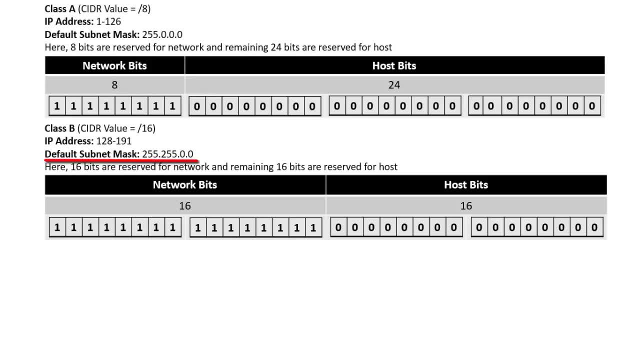 Its default subnet mask is 255.255.0.0 and the default CIDR value is 16.. As we know that the total number of network bits in class B IP address is 16. So its CIDR value is 16.. 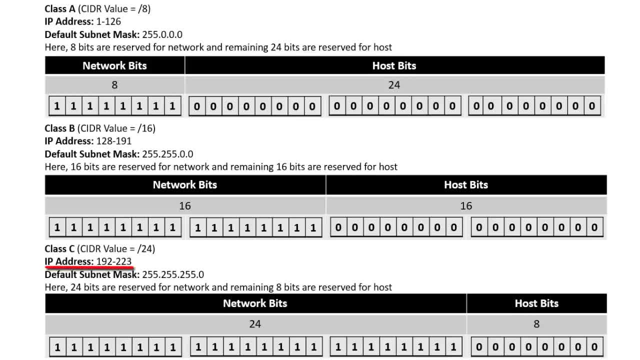 Now let's move on to class C. Class C IP address starts from 192 to 223.. Its default subnet mask is 255.255.255.0 and the default CIDR value is 24.. Now why we have this, Why we have written the CIDR value as 24?. 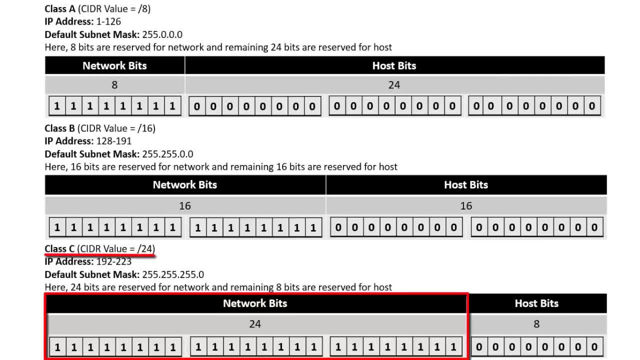 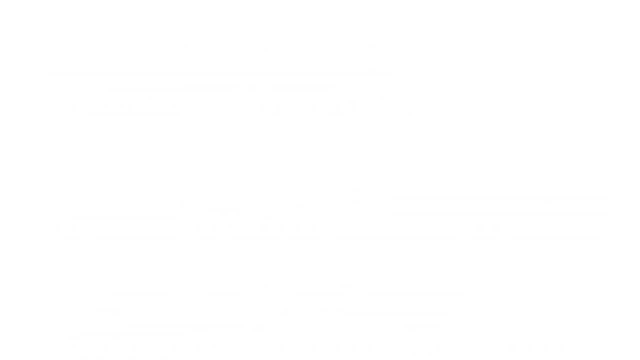 Because total number of network bits in class C IP address is 24.. That is why the CIDR value of class C IP address is 24.. Now let's take an example so that I can clear the concept for you. As here you can see, it's mentioned here: 192.168.10.0, with the CIDR value 24.. Now let's take an example so that I can clear the concept for you, As here you can see, it's mentioned here: 192.168.10.0, with the CIDR value 24.. Now let's take an example so that I can clear the concept for you, As here you can see, it's mentioned here: 192.168.10.0, with the CIDR value 24.. 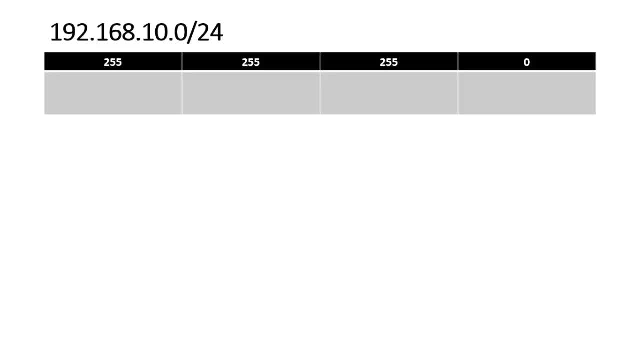 As we know that it is a class C IP address, because the IP address starts from 192 and its default subnet mask is 255.255.255.0.. Now the question is: where does this subnet mask come from? Why the subnet mask of class C IP address is 255.255.255.0?. 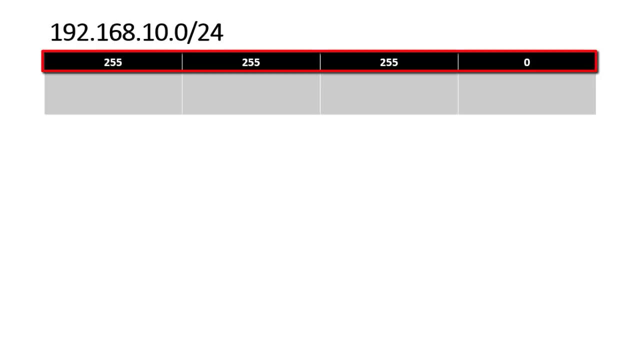 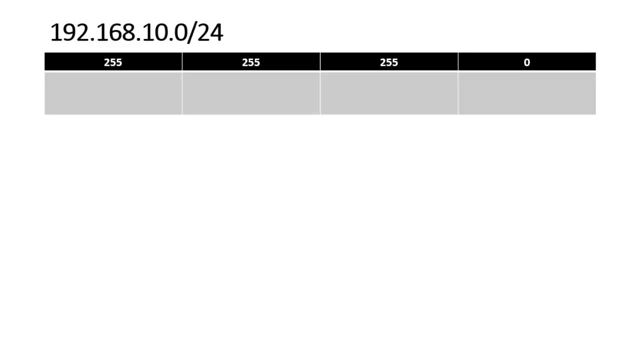 Because we remember that IP version 4 is a 32 bit address and it is divided into 4 blocks of 8 bits, where 1 indicates the network bits and 0 indicates the host bits. Bits on each block count from right to left And it is written as: 2 to the power 0, 2 to the power 1. 2 to the power 0, 2 to the power 1, 2 to the power 1, 2 to the power second and 3 to the power third, and leave two bound units not also. 2 to the power 0, 2 to the power third and leave two bound units not also. And it is written as 2 to the power n at 15Wait for myسalla. Another note: source 2 input are less than 207, ,111,90まあ, which is the memory bred to sum over clip grid or 60s. 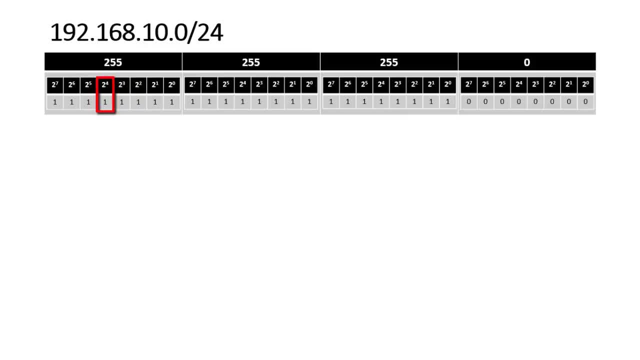 power 2,, 2 to the power 3,, 4,, 5, 6, and 2 to the power 7.. So if you add all these network bits, the total number you will get is 255.. So the default subnet mask of class C, IP. 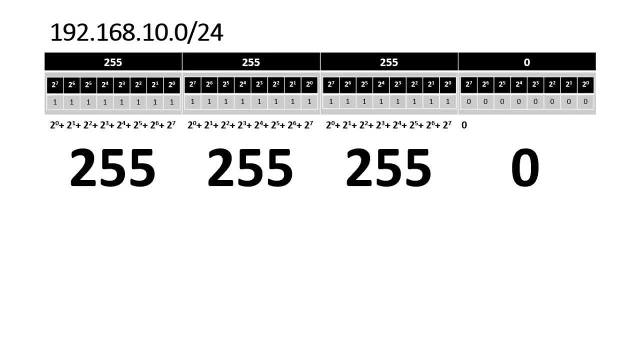 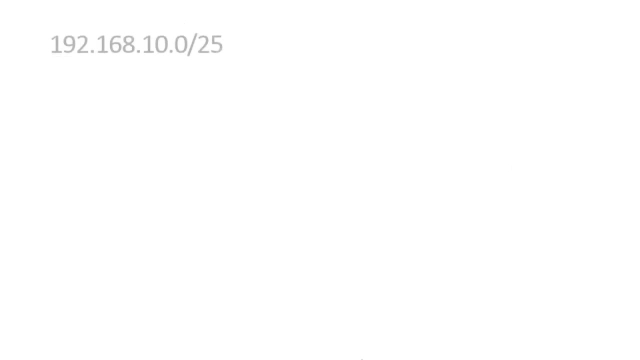 address is 255.255.255.0.. Now why we have written here 0? Because it is a host bit. You can calculate the subnet mask only from the network bit, not from the host bit. That's why we have written here as 0.. Hope the concept is clear for you. Let's take another example. The IP address 192.168.10.0 with the CIDR value 25.. Hence the IP address is same as our previous example, but this time we have changed the CIDR value from 255.255.255.0 to 255.255.0.. So the IP address is 192.168.10.0 with the CIDR value. 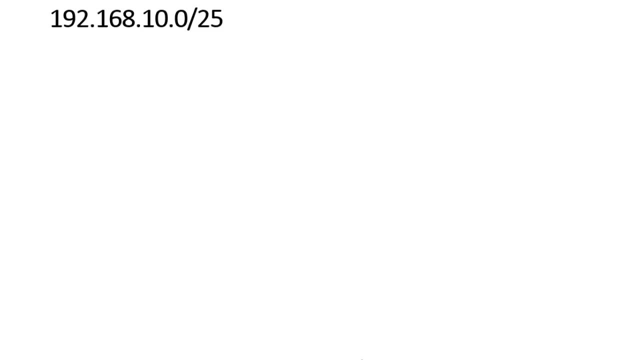 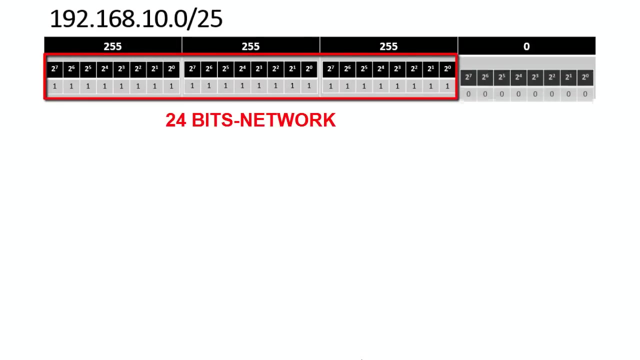 from 24 to 25.. As we know that the default subnet mask of class C IP address is 255.255.255.0. Because by default there are 24 bits reserved for the network and 8 bits reserved for the host, But in this scenario the CIDR value is 25, which means there must be 25 network. 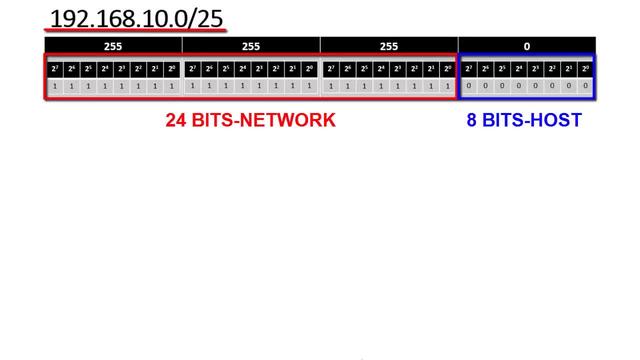 bits. Okay, now the question is: in class C IP address, we are having only 24 network bits. Now from where to find another one bit? The solution is very simple: We have to borrow one bit from the host. So the new subnet mask which you will get is 255.255.255.128.. Now from where do we have? 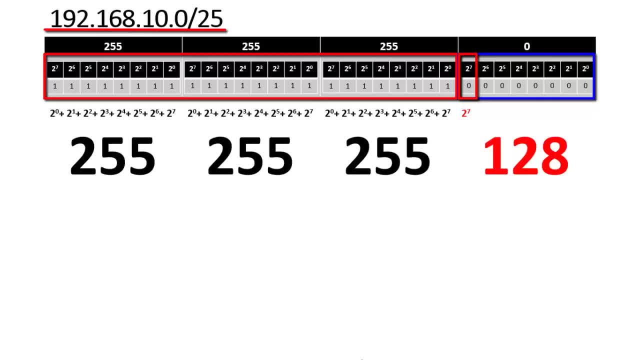 found this 128?? This number came from the network bit which you have borrowed from the host. As here you can see, guys, the value of that particular network bit is 2 to the power 7.. Hence, once you calculate 2 to, 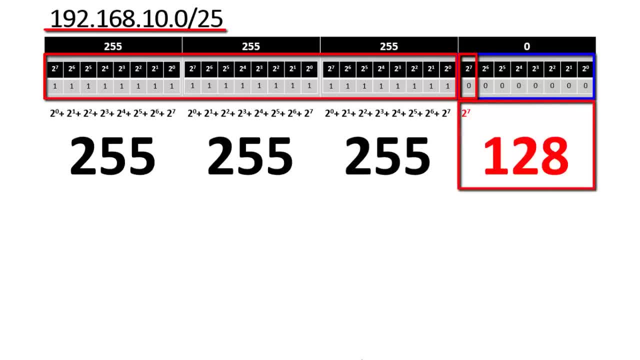 the power 7, the total number you will get is 128.. So for that reason, the new subnet mask of this address is 255.255.255.128.. Is it clear guys? If not, nothing to worry. 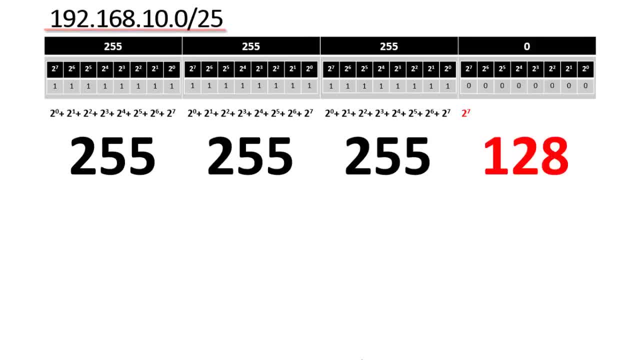 I will also show you another example, But first of all let's look at how to find the number of network from this address. Just follow this small formula 2 to the power n. Here n indicates the total number of bits you have borrowed from the host. Hence, we have borrowed only one bit. 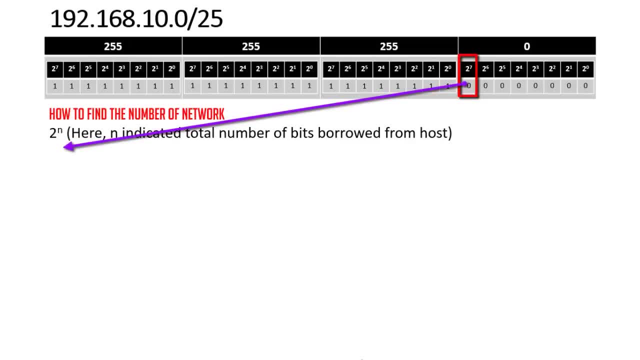 right. So the total number of network you can create is 2 to the power 1,, which is equal to 2. Means only two networks can be created. Now let's find out how to find the number of IP address. 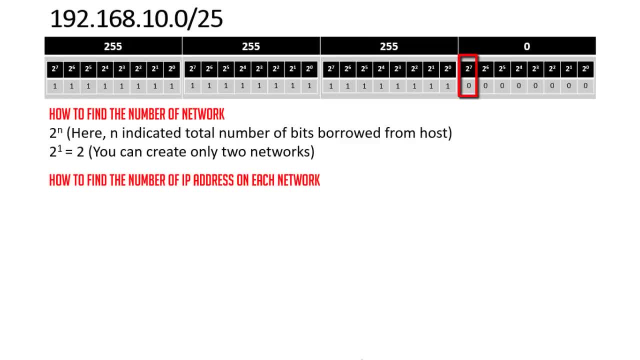 on each network. The formula is very simple. Again, we have to use 2 to the power n, But this time n indicates the total number of host bits. Hence, we have already borrowed one bit from the host. So how do we find the total number of bits you have borrowed from the host? Well, we have. 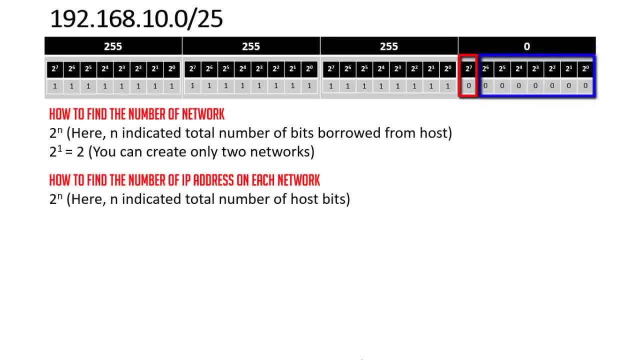 to use 2 to the power n. So how many total bits remaining in the host part? It is 7.. So we are going to use 2 to the power 7, which is equal to 128.. Means on each network you will get 128 IP. 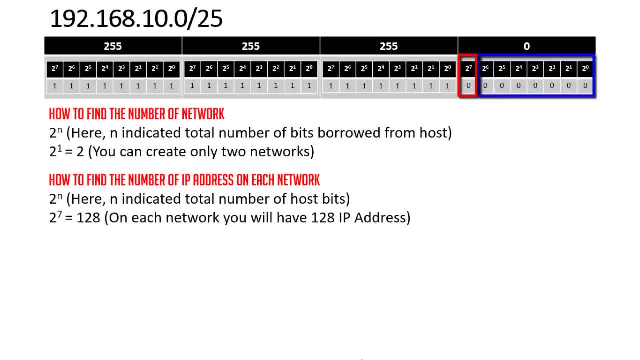 address. Now let's find out how to find the number of hosts on each network. Guys, these two topics are really different: Number of hosts and the number of IP address. Number of IP address means total number of IP address you will get on each network, And number of hosts means total. 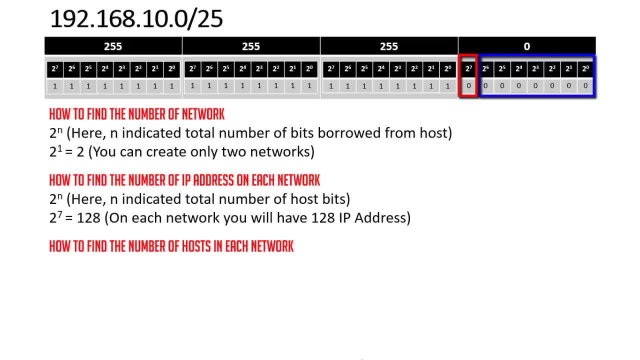 number of IP address you can assign to the devices in a network. So I will explain you that. Hence, the formula is 2 to the power n minus 2.. Here n indicates the total number of remaining host bits, which is 2 to the power 7 minus 2, which is equal to 128.. Now let's find out how to find the number. 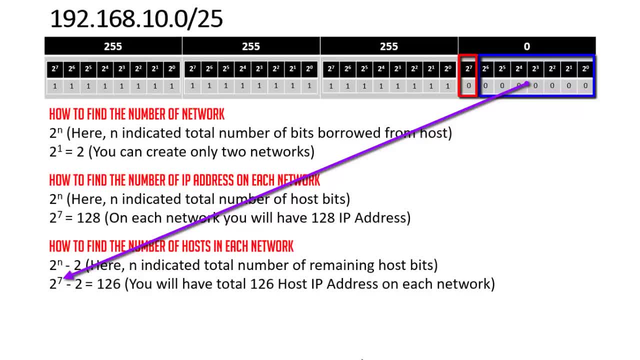 126. It means you will have total 126 host IP address on each network. Means you can assign 126 IP address to the devices in a single network. Now the question is why we have subtract 2 here, Because on every network the first IP address is reserved for the network ID and the last IP. 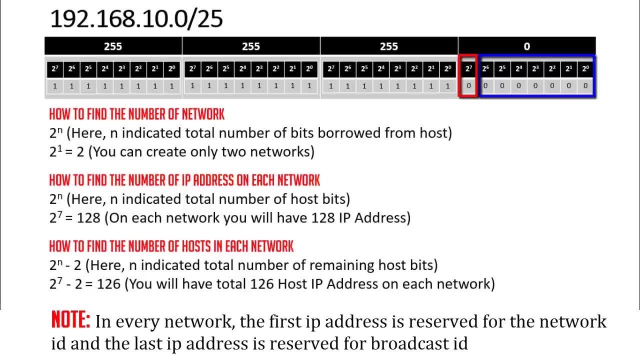 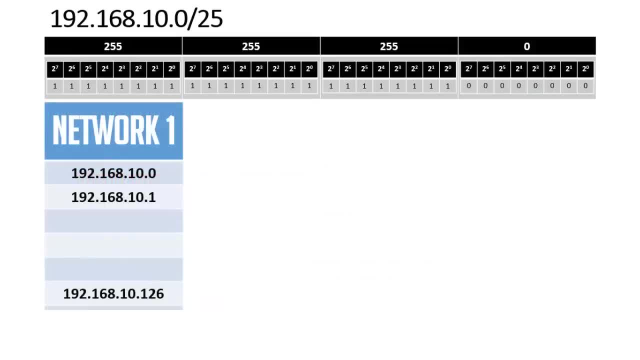 address is a broadcast ID And the last IP address is a broadcast ID And the last IP address is a broadcast ID And these two IP address you cannot use. For this reason, on every network we have to subtract 2.. So as here you can see guys in network 1, the IP address will start from 192.168.10.0. 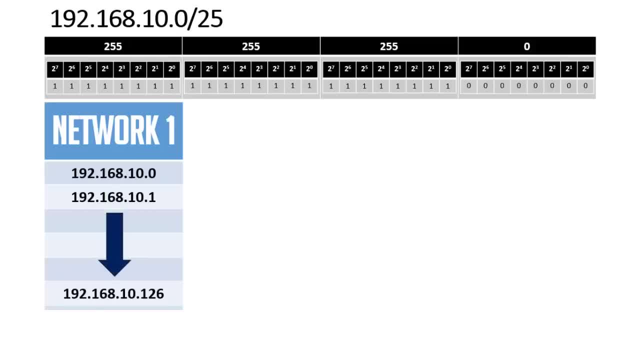 and it will end at 192.168.10.127, which is equal to 128.. Now, as I have explained you, the first IP address is 192.168.10.0.. And the last IP address is 192.168.10.0.. And the last IP address is 192.168.10.0. 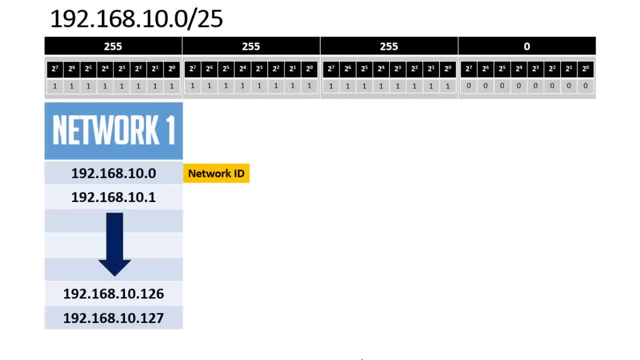 A network ID And the last IP address is broadcast. ID Means these two IP address you cannot use as it is reserved for the network and the broadcast. The IP address which is available at the center of this IP address, that is, from 192.168.10.1 to 192.168.10.126, are the host IP address And this 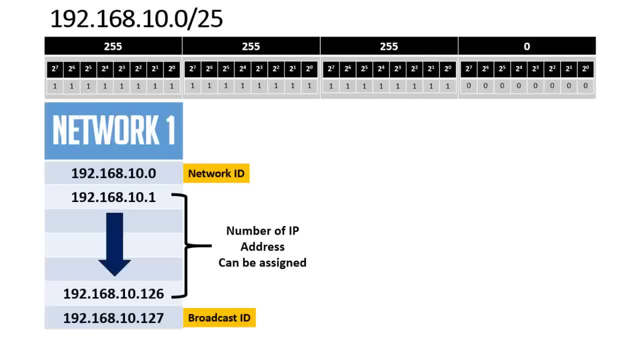 assigned to devices in a network, same like this in network 2. the ip address start from 192.168.10.128 and it will end at 192.168.10.255. hence i have explained you earlier. the first ip address is a. 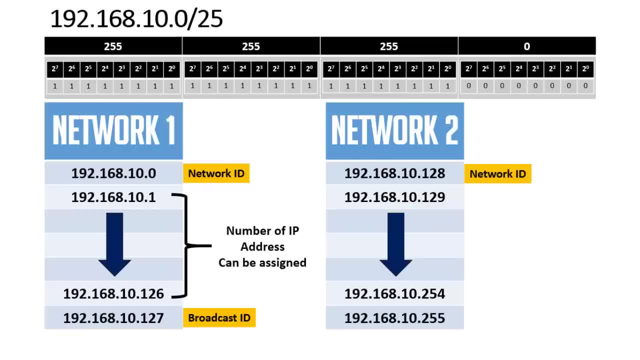 network id and the last ip address is a broadcast id, and the ip address which you are getting at the middle of this are the host ip address, and these ip address start from 192.168.10.129 to 192.168.10.254. these are the ip address which you can assign to the devices in a network. 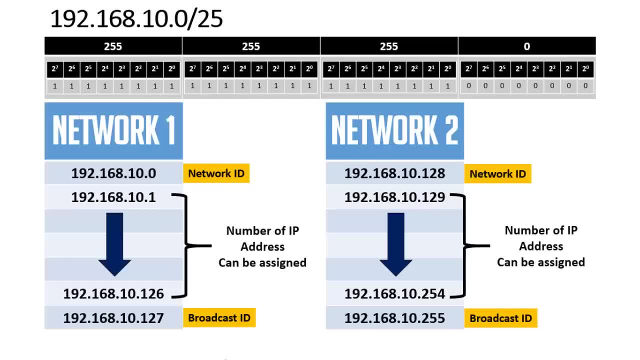 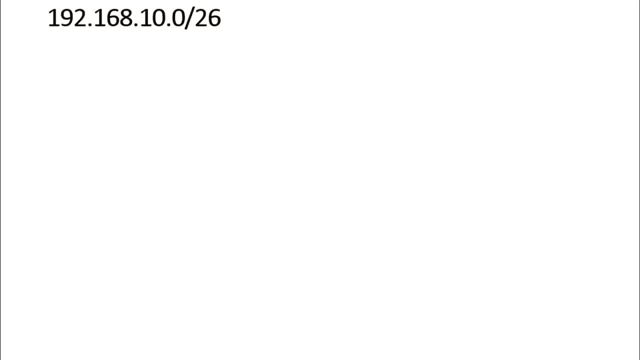 so guys hope the concept is clear. let's take in another example, as here we can see the ip address 192.168.10.255, with the cidr value 26. the ip address is same as our previous example, but this time we are using 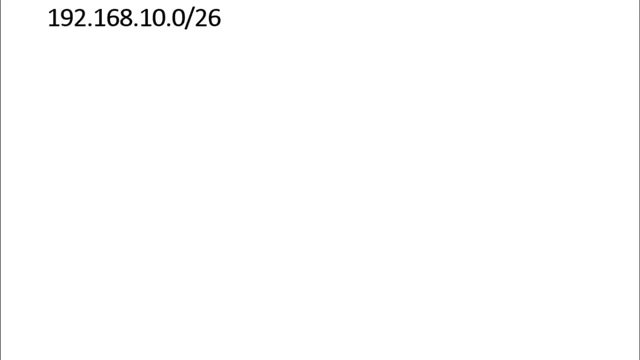 a cidr value 26. as we know that it is a class cip address because the ip address start from 192 and by default the class cip address subject mask is 255.255.255.0. now why the subject mask class cip address is 255.255.255.0. 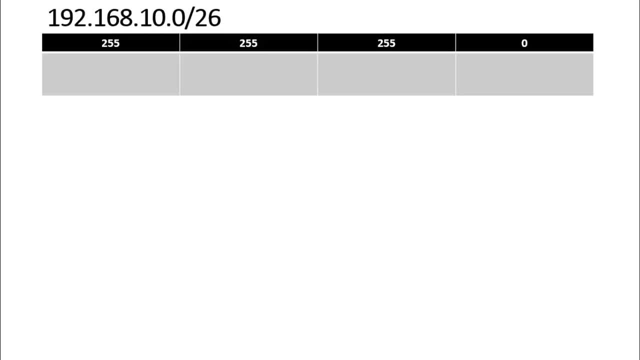 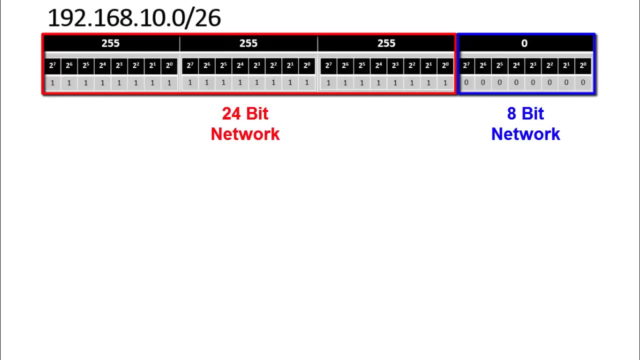 because in class cip address 24 bits are reserved for the network and the 8 bits are reserved for the host. so if you count the value of all these bits on each block you will get the total number of 255.255.255.0. but the question is, the cidr value is 26 and the default network bits on class. 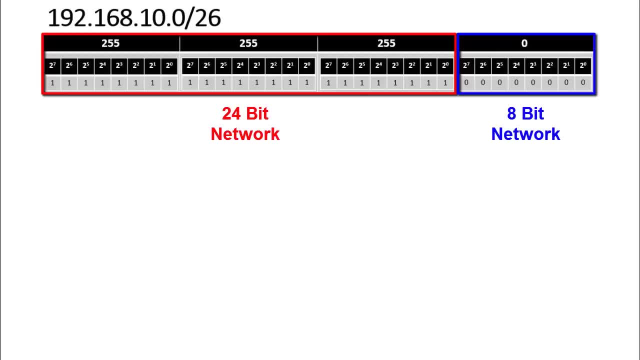 cip address is 24, so from where do we get another two bits? yes, we have to borrow it from the host. so once you borrowed it two bits from the host, the new subject mask, what you will get is 255.255.255.192. 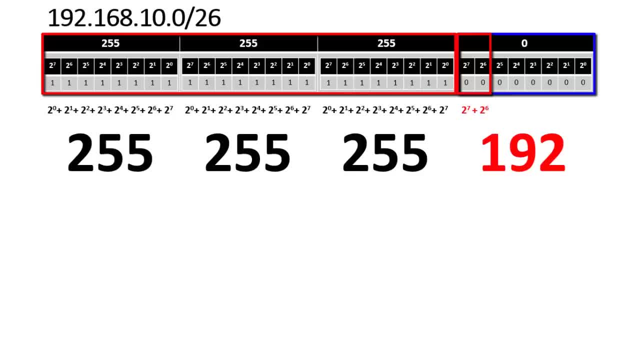 now, how do we get this number 192? because we have borrowed two bits from the host and if you get the bits value, which is two to the power seven plus two to the power six, the total number you will get is 192. so this is how you can find the subject mask. now let's move on on how to find the. 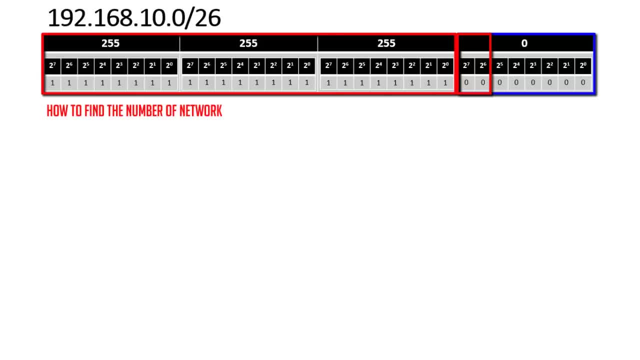 number of networks. the formula is very simple: two to the power n here and indicates the total number of bits borrowed from the host. hence we have borrowed two bits from the host, swagon right two, 2, which is equal to 4. it means you can create total number of 4 networks. 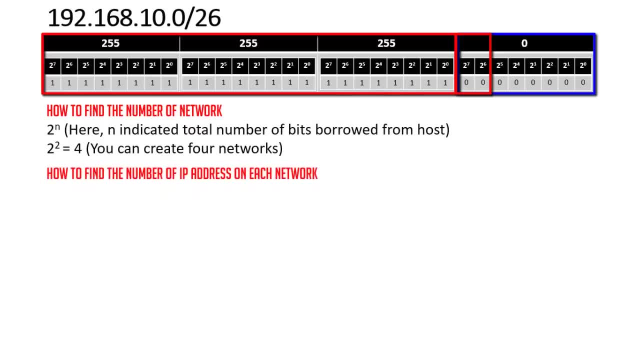 Now the question is how to find the number of IP address on each network. the formula is 2 to the power n, but in this scenario n indicates the total number of remaining host, as We have taken 2 bits to the network. So how many bits remains? 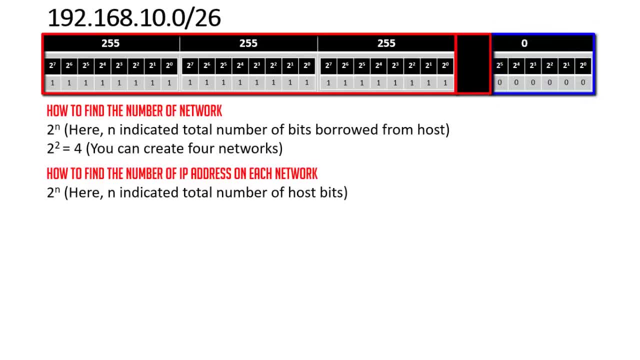 We. it remains only 6 bits, So we are going to write 2 to the power. 6, which is equal to 64. it means you will have 64 IP address on each network. Now let's look at how to find the number of hosts on each network. 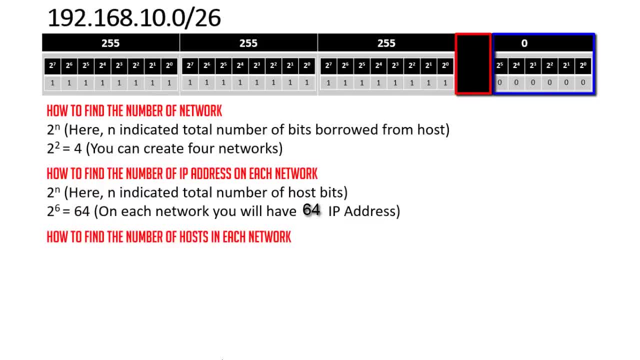 Guys, number of IP address and number of hosts are both different. number of IP address means total number of IP address you will get on each network and Number of host means total number of IP address you can assign to the devices in a network. So the formula is 2 to the power n minus 2. 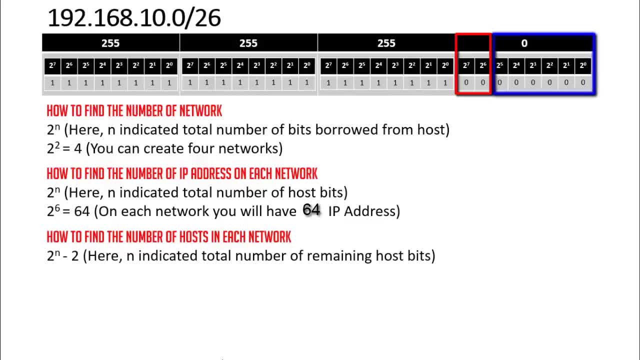 Here: n indicates the total number of remaining bits. Okay, so how many total bits remaining? We have remained 6 bits, So we are going to write 2 to the power, 6 minus 2, which is equal to 62. it means you can. 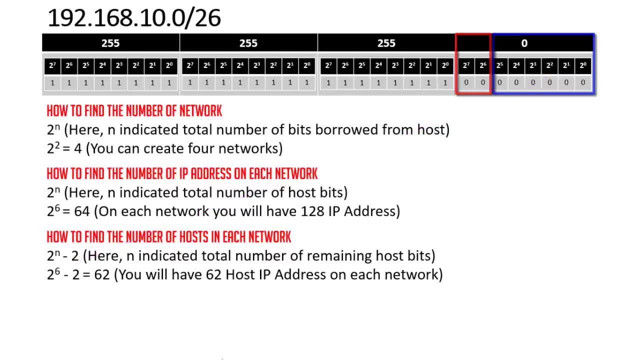 Assign 62 host IP address on each network. Now the question is, why do we have subtract 2 here? right, We have subtract 2 here because on every network The first IP address is reserved for the network ID and the last IP address is reserved for the broadcast ID. and these two 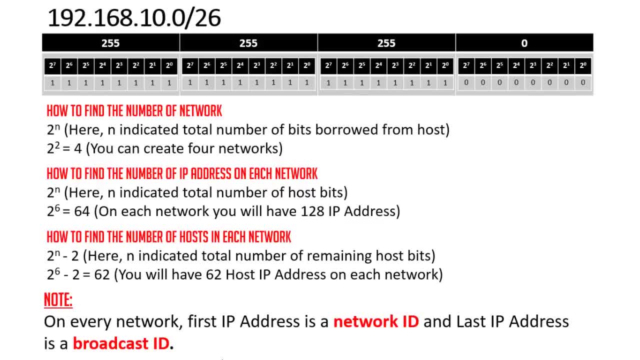 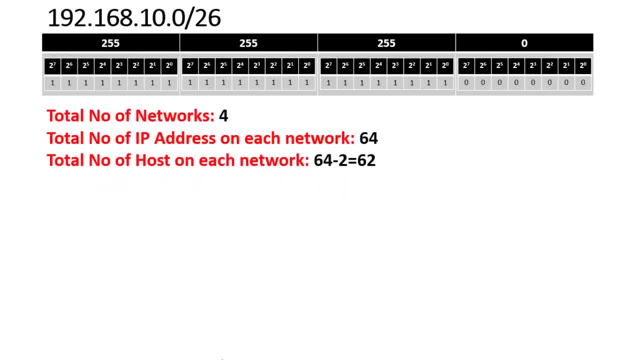 IP address you cannot use. Hope the concept is clear. So the total number of network we have four. total number of IP address on each network is 64 and the total number of hosts on each network is 62, so hence we have four networks. So let name this network as. 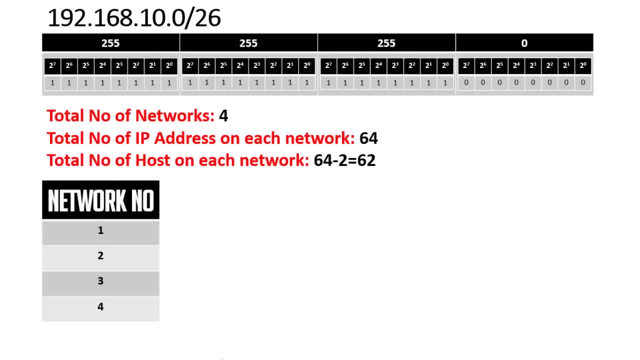 Network 1, network 2, 3 and four. now how to find the network ID for this? We have to just keep adding 64, 64, 64, 64, So like that you can easily find the network ID. So the network ID of first network will be: 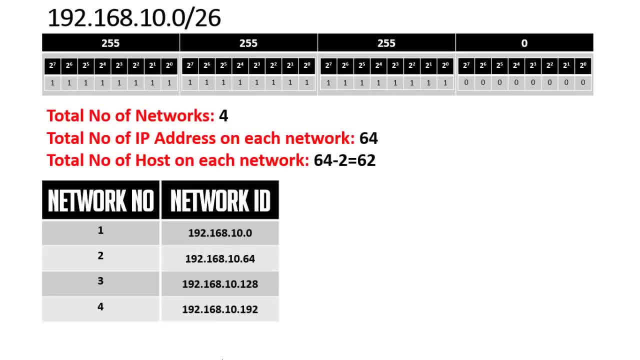 192.168.10.0 and the network ID of second network will be 0 plus 64. how much it is 64. so it will be 192.168.10.64. Now the third network network ID will be 64 plus 64. 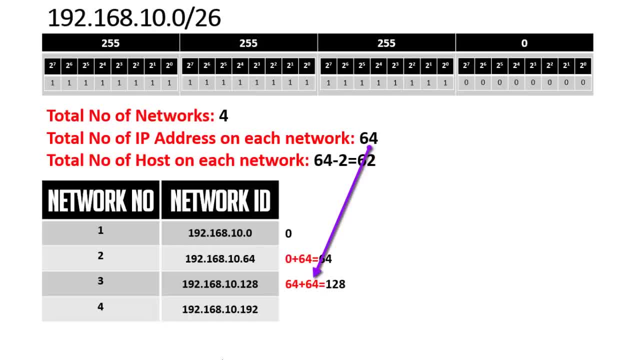 128, so it is 192.168.10.128. Now, what will be the fourth network ID? It will be 128 plus 64, which is equal to 192. so the network ID of fourth network is 192.168.10.192. 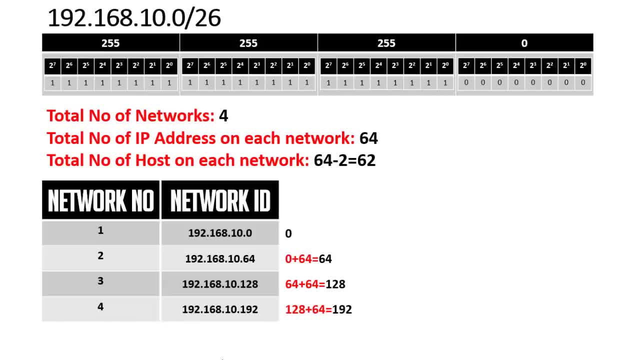 So this is how you can find the network ID. Just you have to add the total number of IP address on each network And you will find the network ID easily. Now let's find the total number of host and the broadcast address. Hence our IP address start from 192.168.10.0. 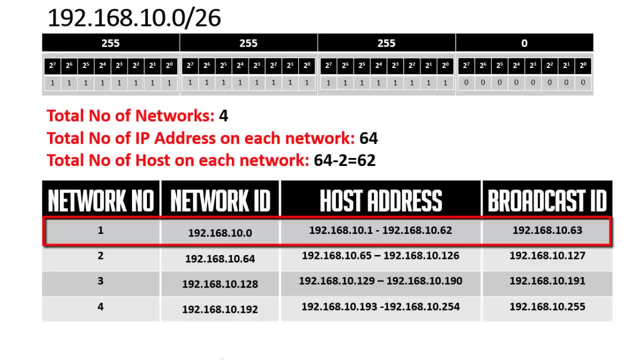 So its host definitely start from 192.168.10.1 to 192.168.10.62 And the last IP address, which is broadcast address, is 192.168.10.62 And the last IP address which is broadcast address is 192.168.10.63. 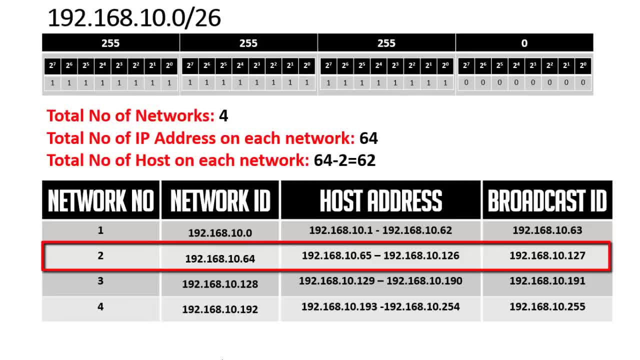 Same in network 2. the first IP address is 192.168.10.64, Which also called network ID, and it will, its host, start from 192.168.10.65 and it will end at 192.168.10.126 and it broadcast address will be. 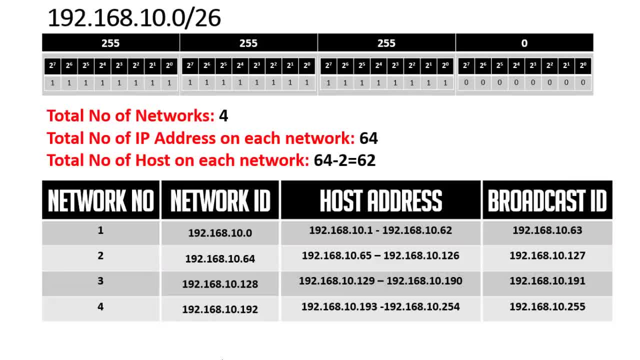 192.168.10.127. What is broadcast address, guys? the broadcast address is the last IP address of each network, Same. you can see the third and the fourth network. So, guys, hope the concept is clear for you If you are having any doubts or want me to make another video on subnetting. 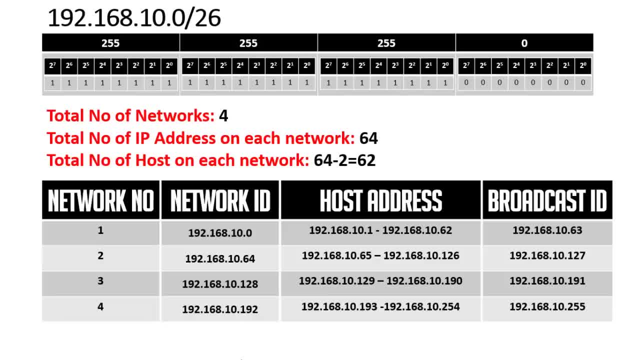 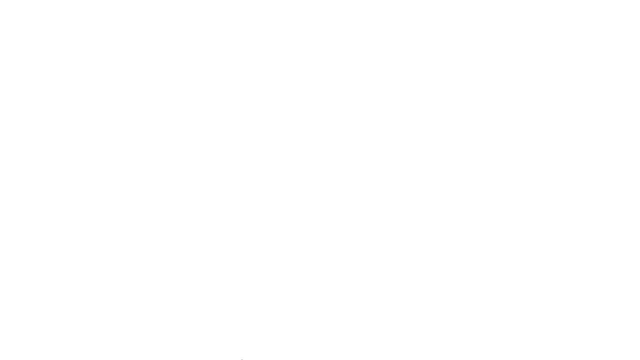 Please let me know in the comment section below. with that, you can also download our Android application Networking plus from the Google Play Store, and also you can download it from from the link given in the description section below. now it's time for the test, so here i'm going. 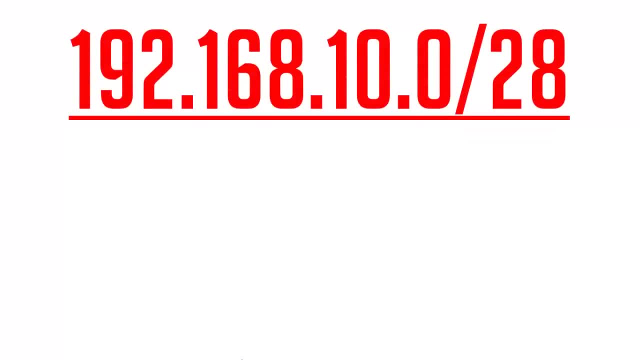 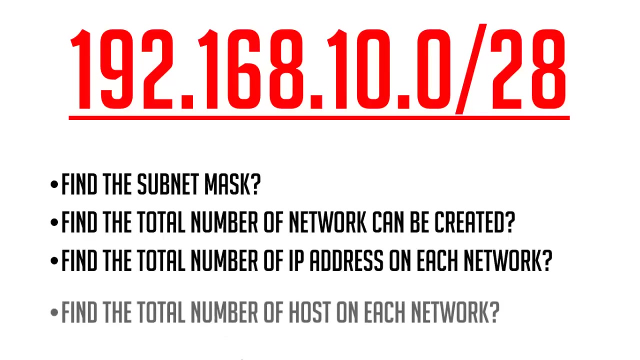 to ask a small question. it is 192.168.10.0 with this area value 28. now tell me, guys, what will be the subnet mask for this. find the total number of network can be created from this. find the total number of ip address on each network. at last, find the total number of host can be assigned on each.